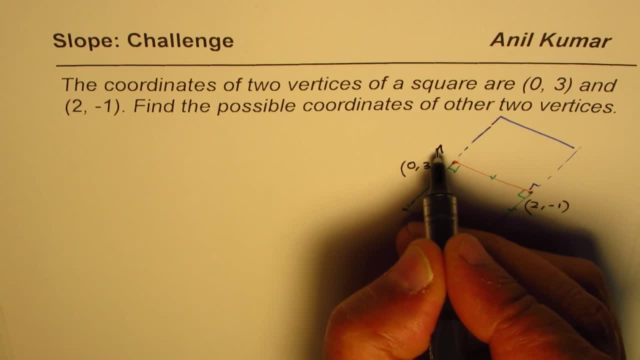 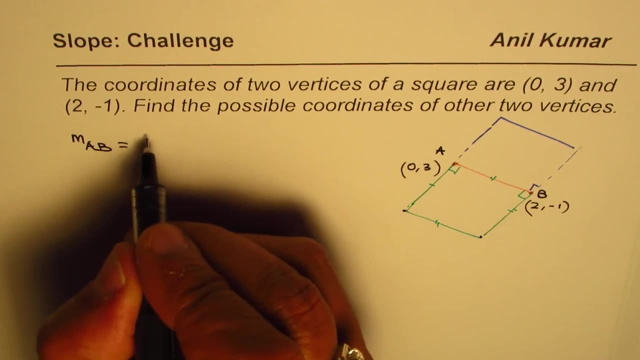 or they should be negative. 2. They should be negative, reciprocal. So let me call these points as a and b. So let's find the slope a- b. first Slope of a and b is y2 minus y1 divided by x2 minus x1,. 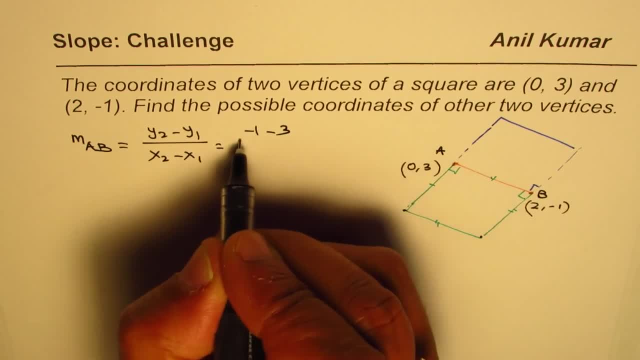 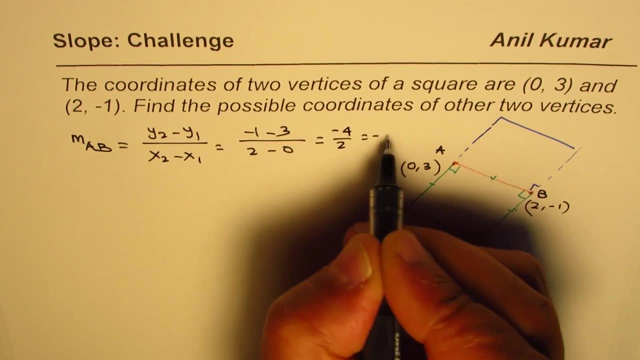 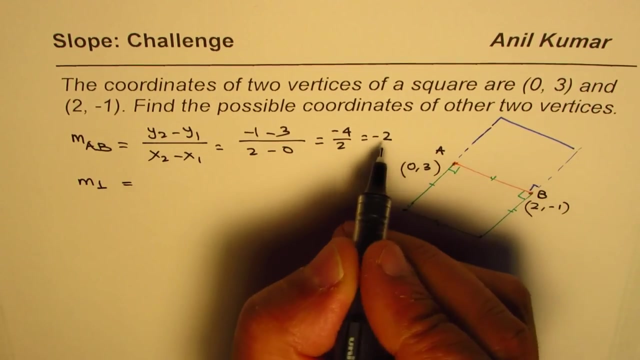 which is minus 1 minus 3 divided by 2 minus 0, or minus 4 divided by 2 or minus 2.. Aligned perpendicular to this, we'll have slope of. let me write perpendicular line: negative reciprocal. that is half correct. 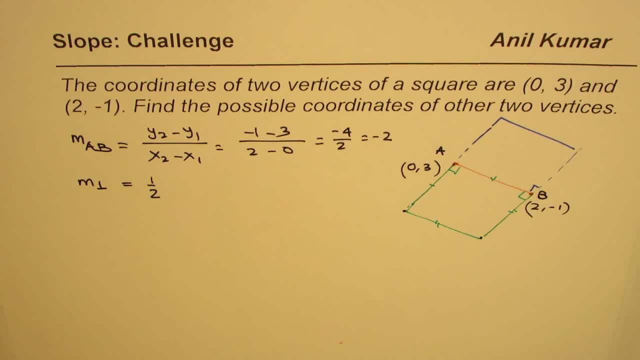 So that is the slope half. Now, another way of looking into this question is that if I move from a to b, then, really speaking, what is the change in x and what is the change in y? right, This is what we wrote here. 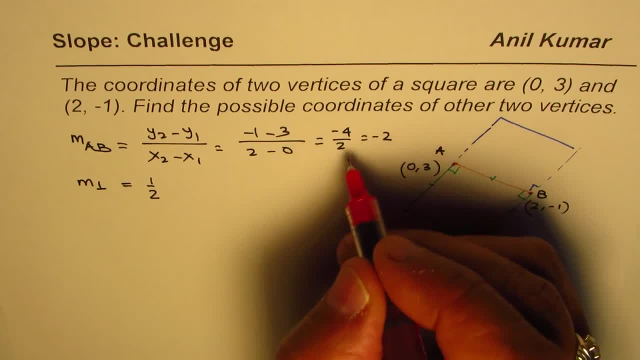 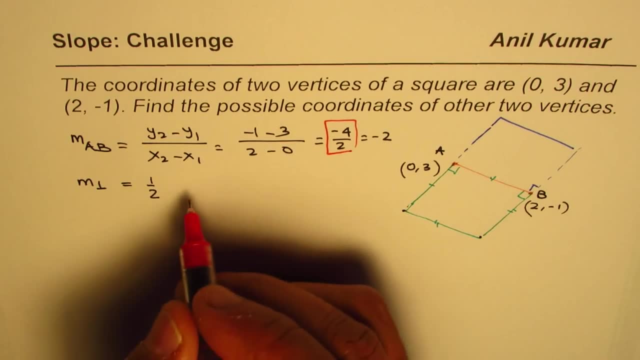 So it is minus 4 over 2.. So let's concentrate on this: Minus 4.. Minus 4 over 2.. So when I say half, in that case it could be like 2 over 4, is it okay? 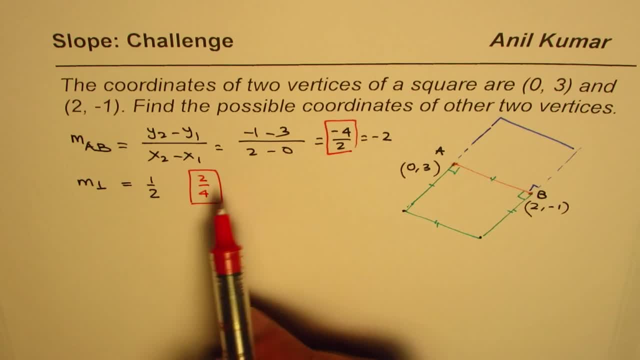 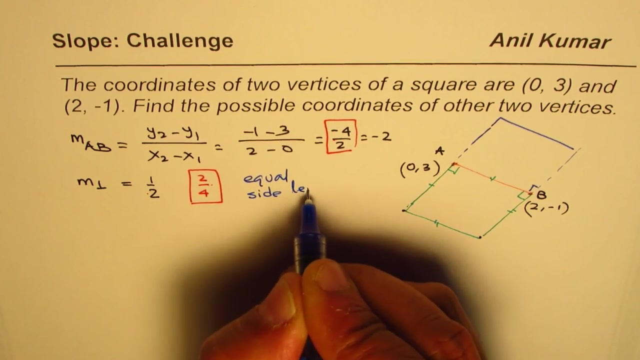 The change could be 2 over 4.. So if I maintain this constant change, this is a ratio. If I maintain this, then I also ensure equal side lengths. right, So that means equal side lengths. So this is a very important concept to understand. 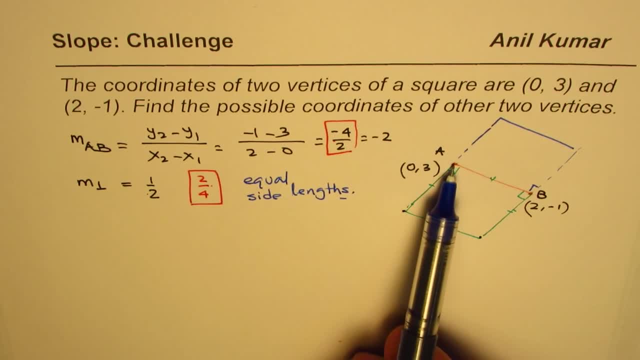 That is to say, if I add minus 4 to y and 2 to x value, I'll get that coordinate of b. But if I do, if I add 4 to x value and 2 to y value, I'll get coordinates of the other vertex from a. 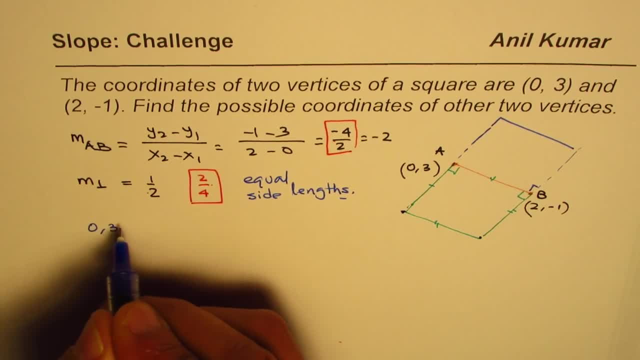 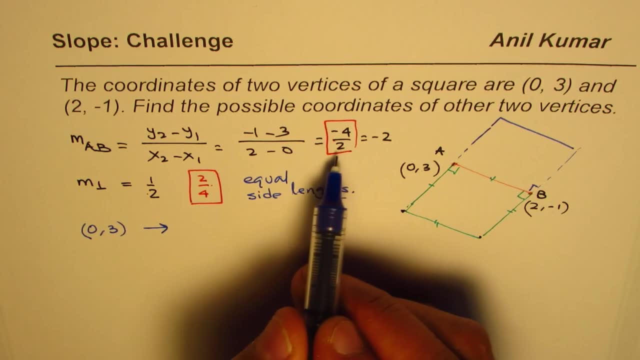 Do you see that? So, starting from a which is 0,, 3,, if I do, 4, so instead of going, we are going 2 right 4 down. Do you see 2 right 4 down? 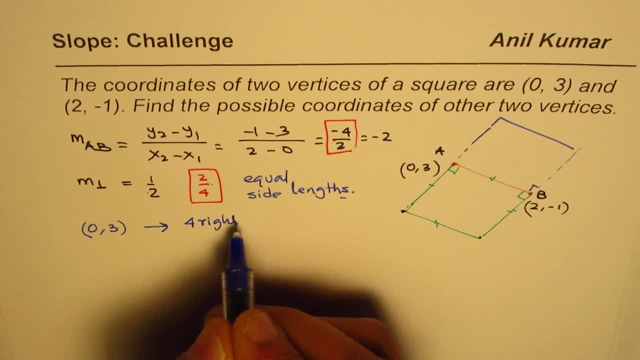 If I, instead of that, we go 4 right 2 up, then where will we reach 4 right 2 up right? So if I do 4 right 2 up, then 4 gets added to 0.. 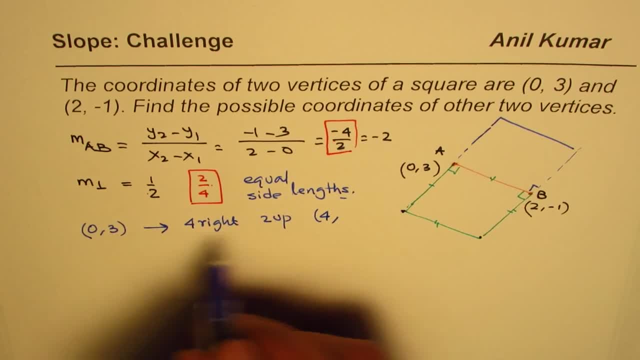 So we get 4 here and 2 gets added to 3. So we get 5.. So in fact we go 4 right, 2 up. we'll come to this point. So it is this point. 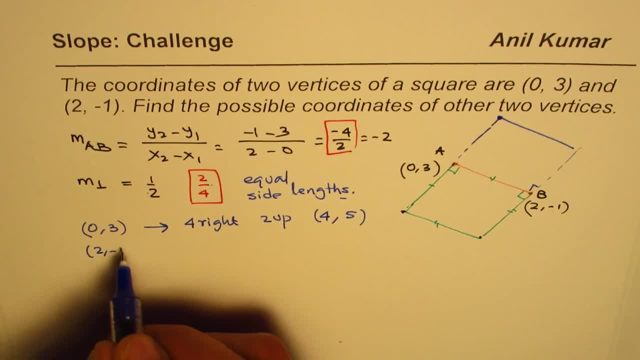 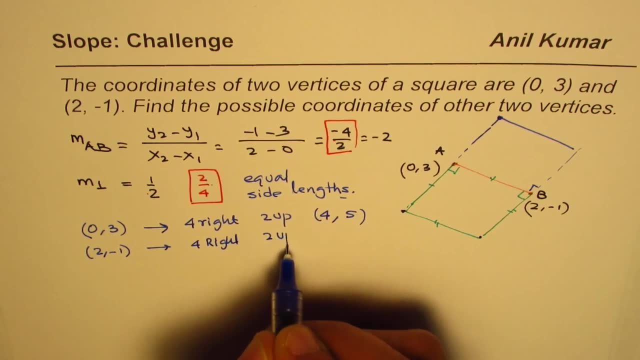 Similarly, from b, we have the point 2 minus 1.. If we do 4 right 2 up, 4 right 2 up, in that case we'll add 4 to the x value, which is 6.. 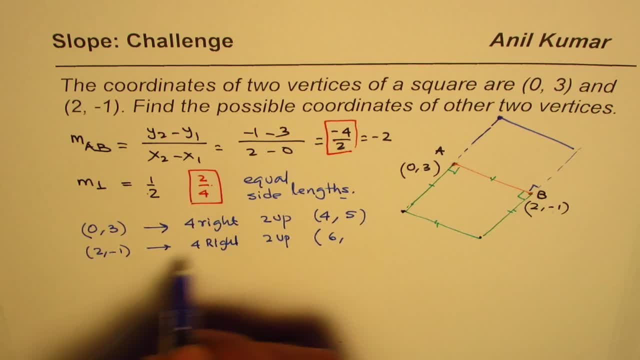 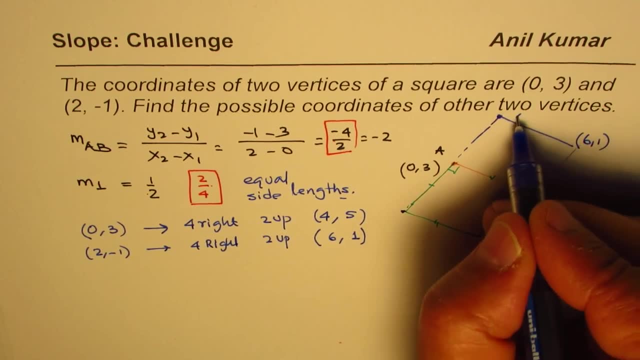 2 up means add 2 to the y value. Minus 1 plus 2 will give us plus 1.. Do you see that? So we get a point here which is 6, 1, and that point will be 4, 5 for us. 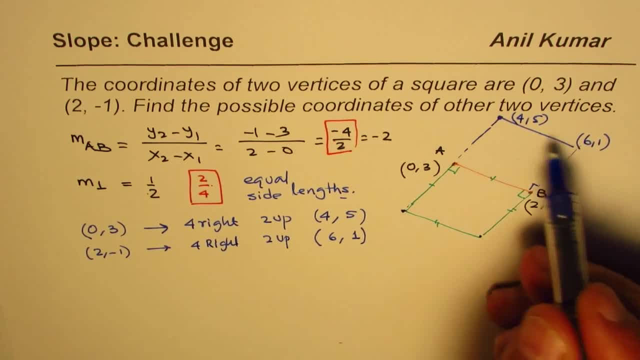 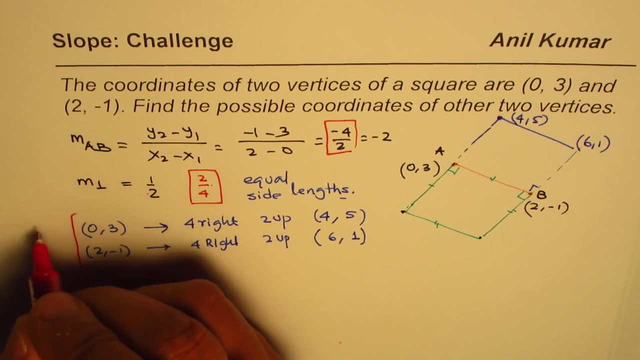 So that is one set of points which will form a square with the given set of points. So this is one solution. So let me call this as solution 1,. okay, Now let's find the second solution, right. 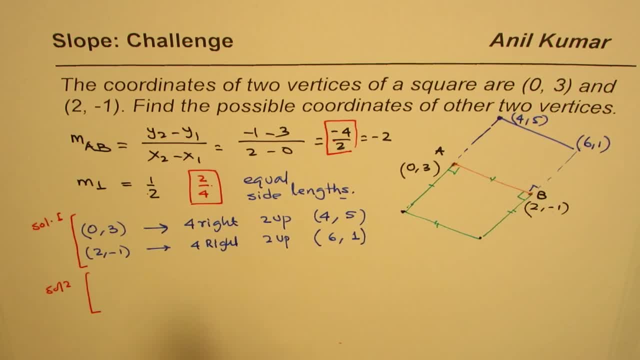 So in the second solution, what are we trying to do? Instead of moving right and up, we'll move left and down right. Both negative will also be positive. That's the whole idea. So 0, 3 will show 4 left, 2 down. okay. 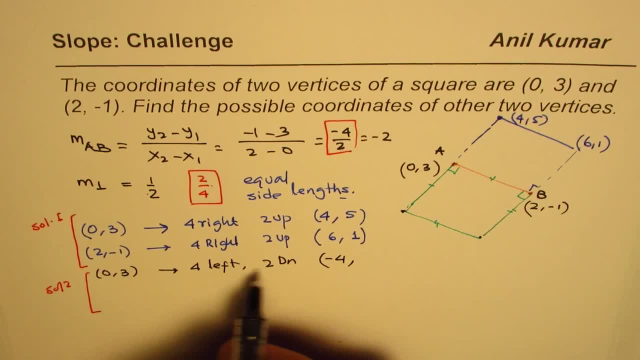 That means left means take away, take away 4, and 2 down means take away 2.. So we get 2 minus 4, 1. Starting with 2 minus 1,, 4 left, 2 down. 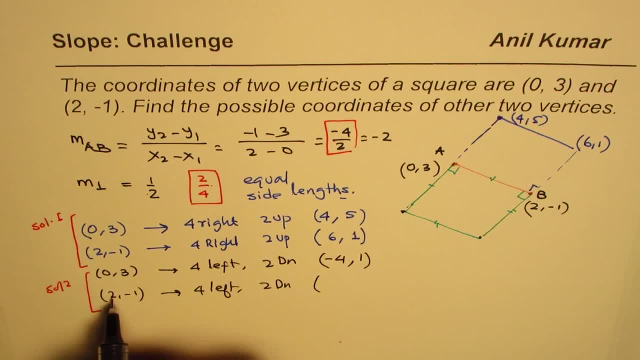 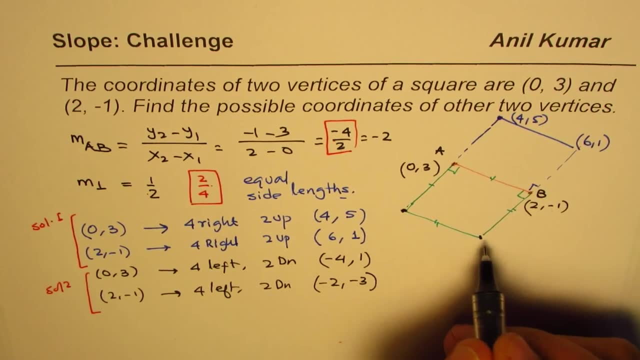 2 down will really means left means take away 4,, that is minus 2.. 2 down means minus 2,, so that means minus 3.. So these coordinate points will be minus 4, 1, and minus 2, minus 3..